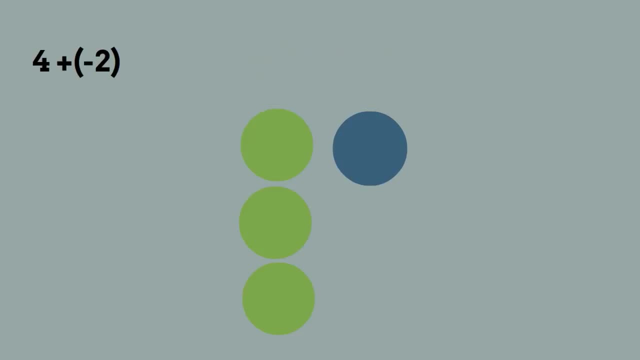 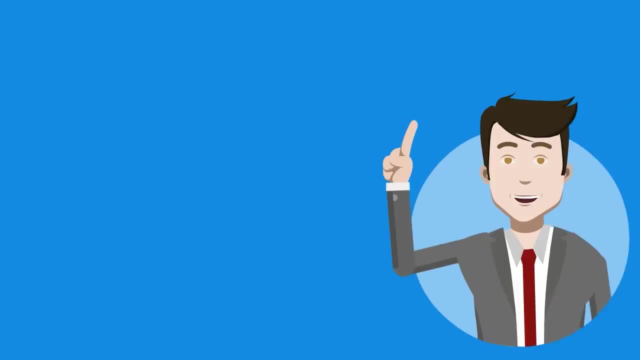 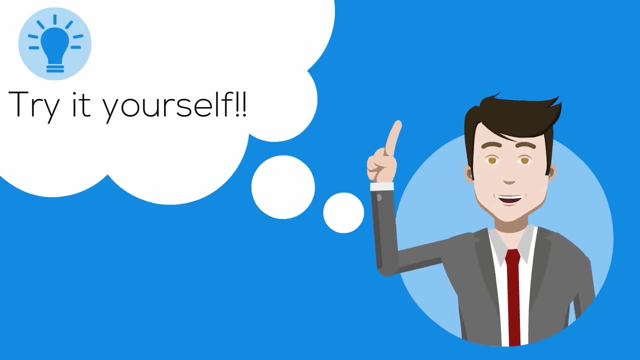 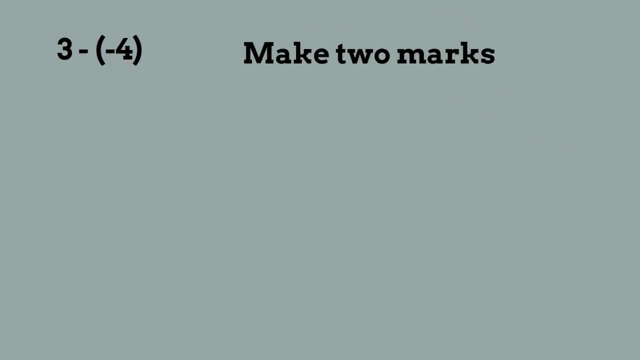 Cancel out your zero pairs. Here they go And you are left with two positive counters. So the answer is positive two. So you want to note that when you're kind of picking the right ones. Okay, I want to show you how to subtract four positive entries. 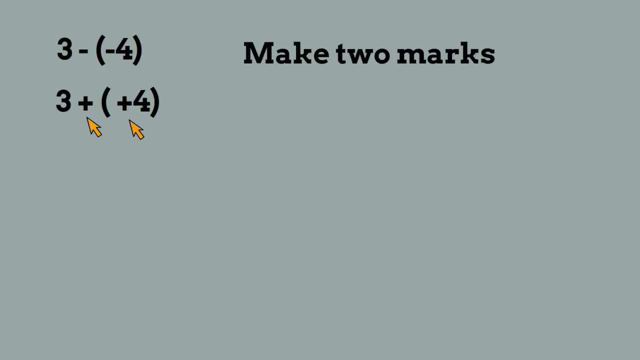 So you can go ahead and try it yourself. You can use just about anything as counters. An easy way are pennies and nickels. Now the rules for subtracting are a little bit different, and I'll leave a link for a 4 to a positive 4, and then you just add like you normally would. 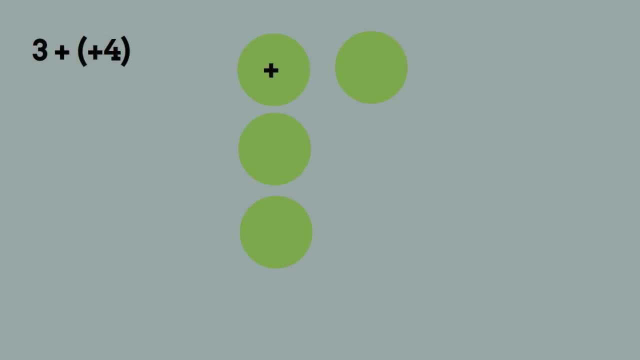 So now let's put the counters down. We'll put 3 positive for the positive 3, and then we put 4 positives for the 4, and that gives us 7 positive numbers total. Let's apply the two mark rule to another problem. 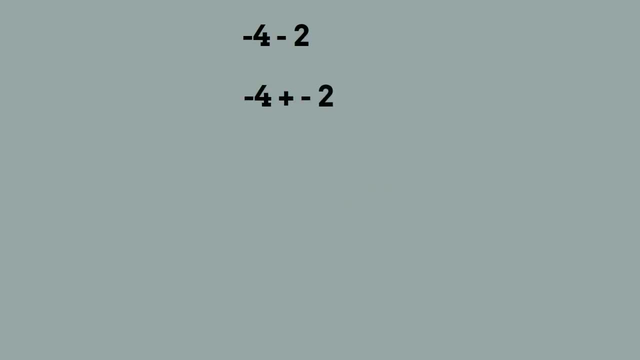 You have negative 4 minus 2.. You apply the two mark rule. The subtraction becomes a positive and then the positive 2 becomes a negative 2. Now we just add it, like we normally would. So now we put the negative counters down, so we have negative 4 and then we have negative. 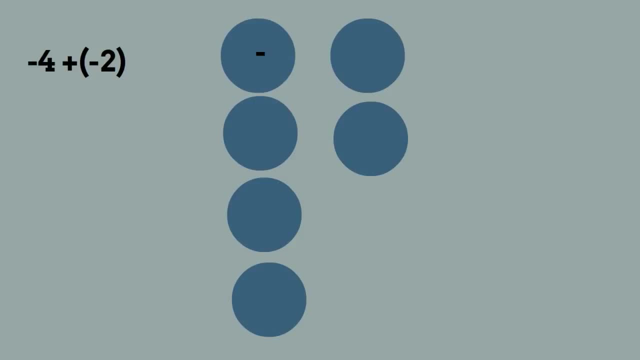 2, and that gives us a grand total of negative 6, because we have 6 negative markers For this problem. we have negative 2 minus 2. Minus a negative 3. Apply the two mark rule: The subtraction becomes addition and the negative 3 becomes a positive 3.. 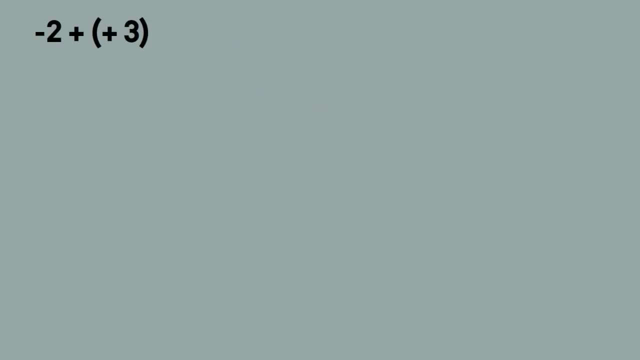 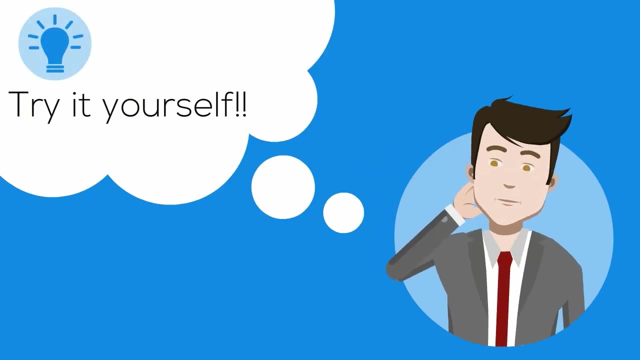 And then let's add, Let's put down two negative counters and then three positive counters, Get rid of the zero pairs and we are left with a positive 1.. Thank you, So go ahead and try it yourself. Apply the two mark rule to subtraction. 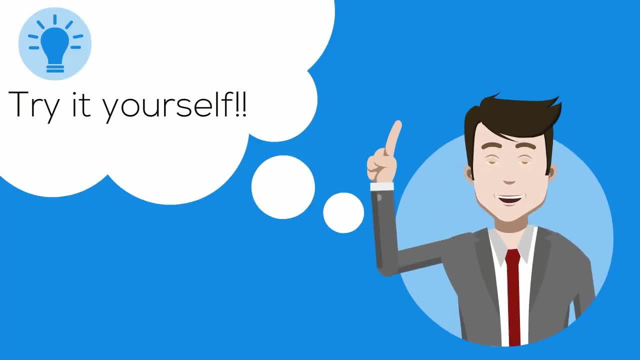 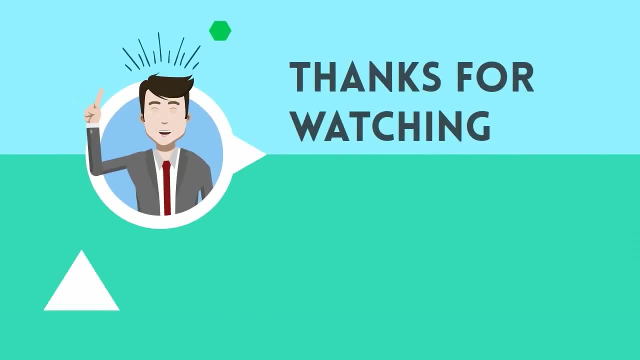 It converts the subtraction sign to a plus sign and then reverses the sign of the other number and then you just add normally Thanks for watching, and MooMooMath and Science uploads a new math or science video every day. Please subscribe and share.